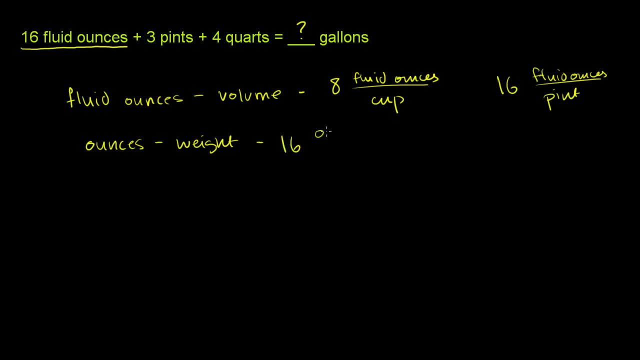 Ounces, which is a unit of weight, you have 16 ounces per pound, And since I told you that a fluid ounce is a little bit more than an ounce, you could kind of figure out that, hey, a pint of water at standard temperature and pressure, and all of that. 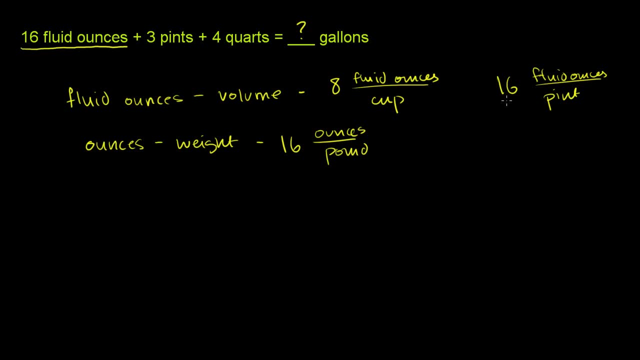 that a pint of water will weigh a little bit more- Almost a pound, or actually a little bit more than a pound, but roughly equal to a pound. So that's something that might make things simpler or more difficult. Now let's actually tackle the problem. 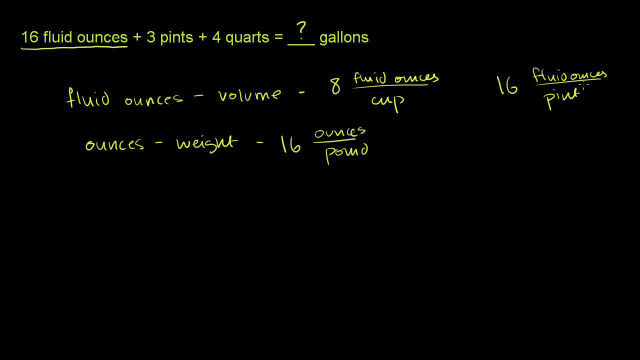 So we have 16 fluid ounces. I just told you that there are 16 fluid ounces per pint, So 16 fluid ounces. let me write it over here. So 16 fluid ounces- Fluid ounces times. Now we want the fluid ounces to cancel out. 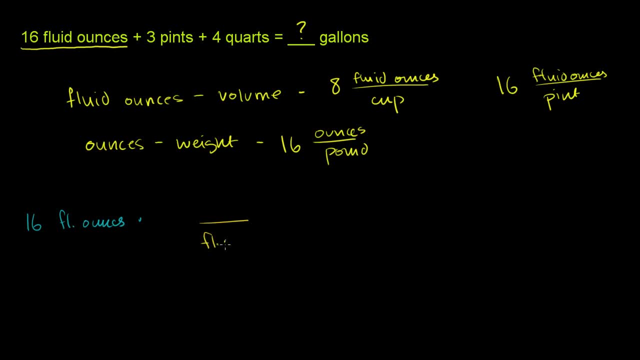 So we want fluid ounces in the denominator Times: fluid ounces. Now, how many fluid ounces are there per pint? We want a pint in the numerator so that this and this cancel out. Well, we just saw that there are 16 fluid ounces per pint. 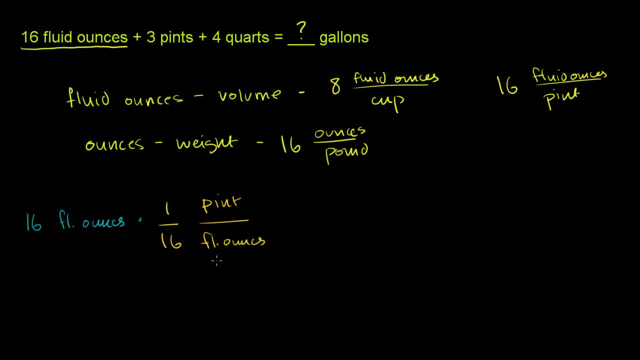 or that 1, 16th of a pint per fluid ounce, Either way, But we see this and this will cancel out. And so 16 over 16,. this is 16 times 1. divided by 16, is equal to 1 pint. 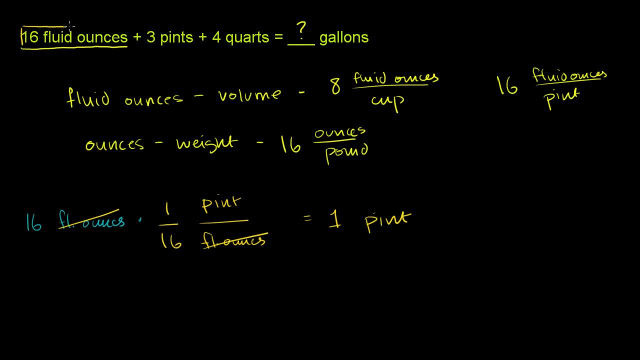 And we know that 16 fluid ounces is equal to a pint. If we have 16 fluid ounces right over here, this is 1 pint right over there. So we have 1 pint plus another 3 pints. So if we were to add all of this part right here together, 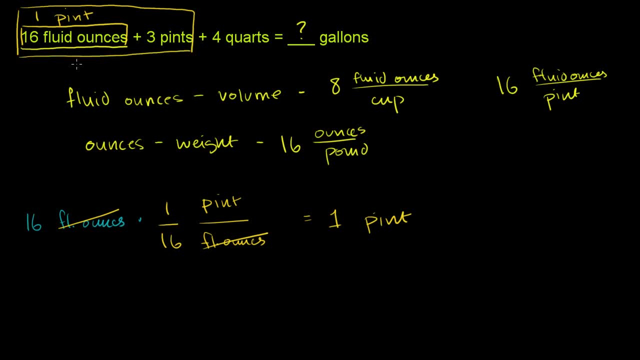 if we were to add all of that together, 1 pint plus 3 pints is 4 pints, 4 pints. Now we have 4 pints. Let's convert it to quarts: 4 pints. 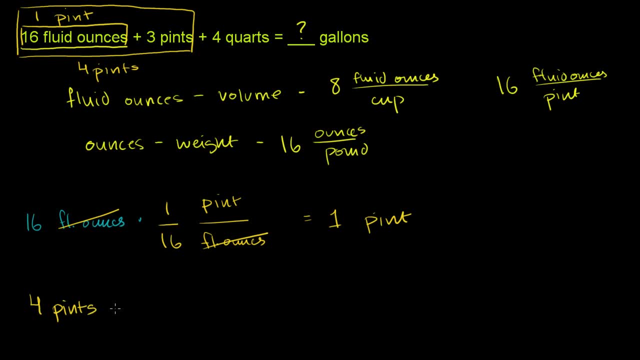 Now we know that there are 2 pints per quart, Or we could view it this way: We want the pints to cancel out, Or 1 quart is 2 pints, Or 1 half quart per pint, And we wrote it this way.